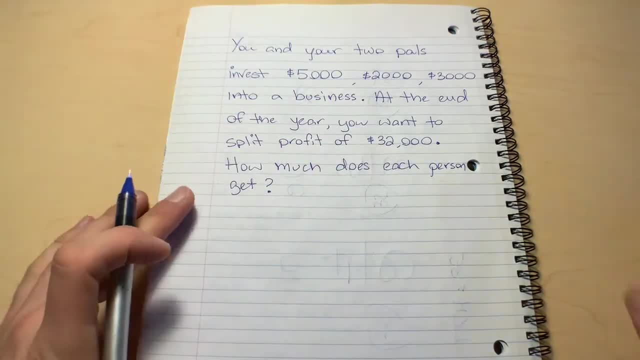 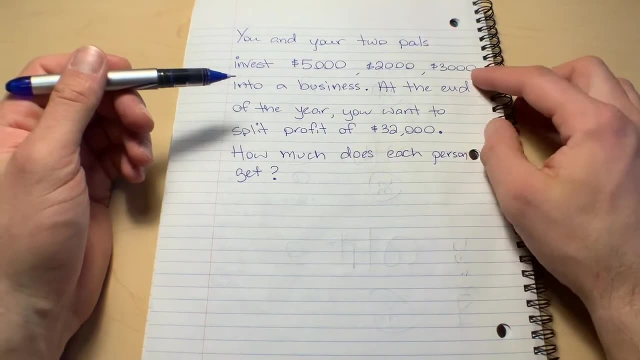 still split up the profits Okay. so the easiest way to do that is to first ask the investor: how much does each person get? How much does each person get How much does add up the values of all of the investments? So if we add up those values, we get $5,000 and $2,000. 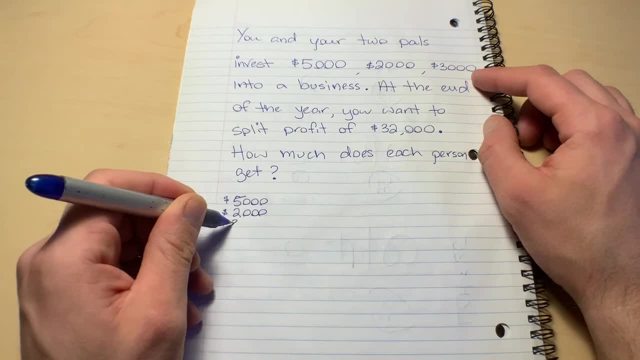 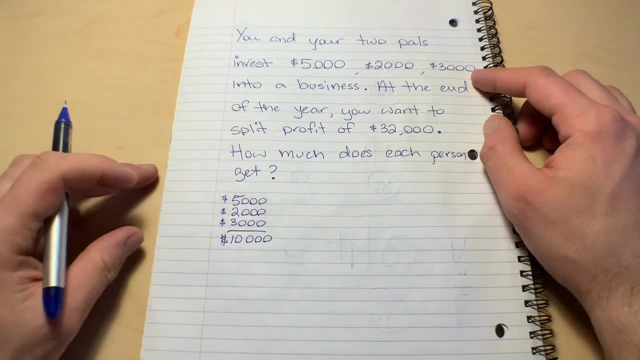 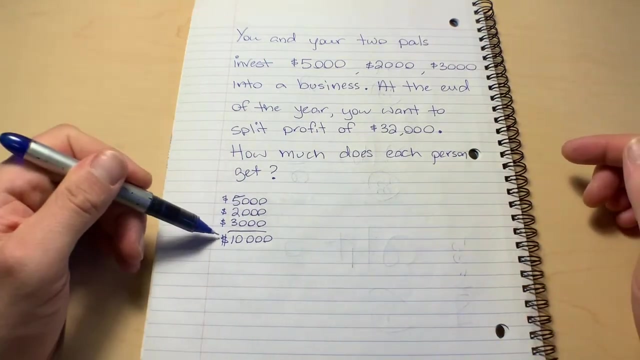 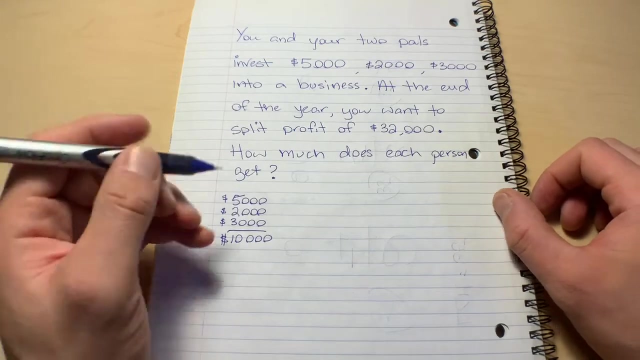 and $3,000.. That's going to give us $10,000.. Blam $10,000.. Okay, so basically, the total investment into this business is $10,000.. We want to split profit of $32,000.. So what we're going to do is take our profit of $32,000. 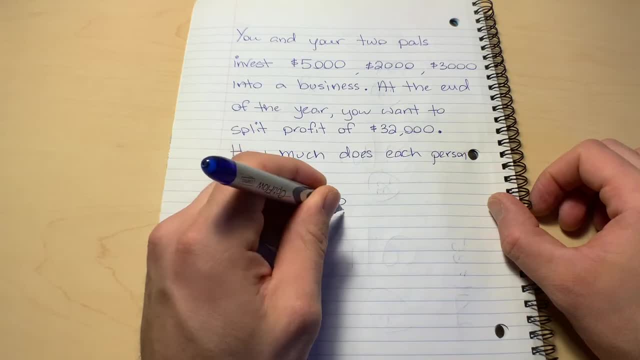 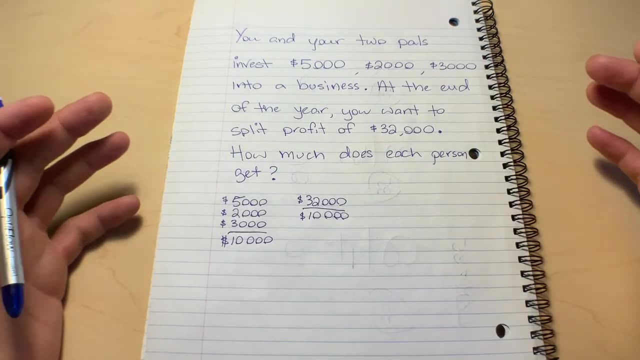 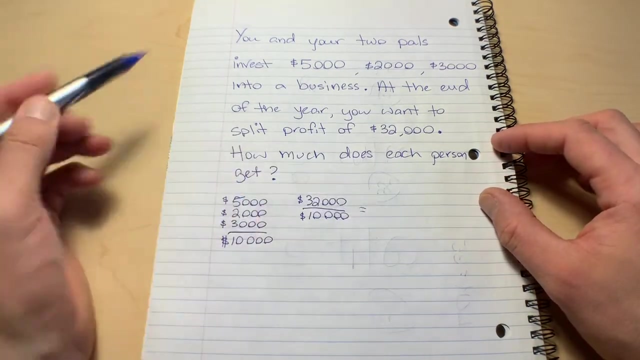 and divide it by all of the investment dollars. Now you guys know from when we did per unit calculations that when you divide this you're going to get an answer Okay. so if we divide this we get an answer like 3.2.. 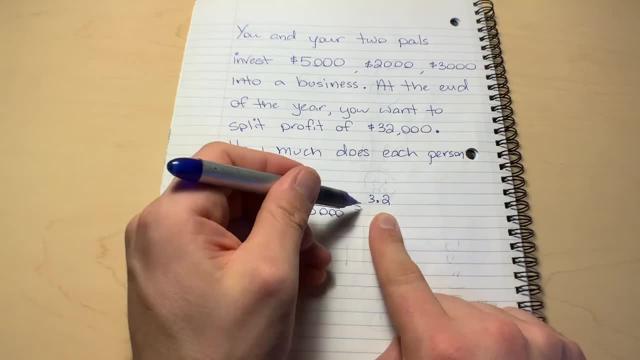 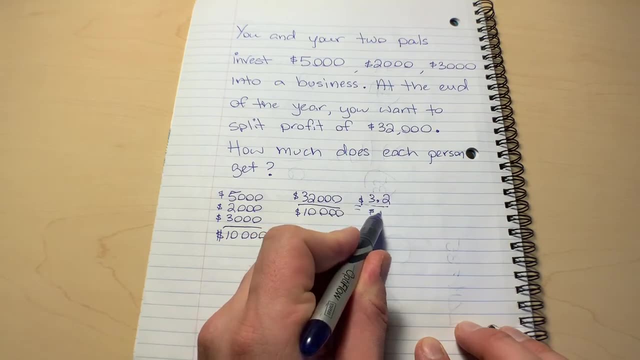 So that means 3.2 is $3,000.. So if we divide this we get an answer like 3.2.. $3.2 for every $1, oops, $1- of investment right. So we're keeping the investment dollars. 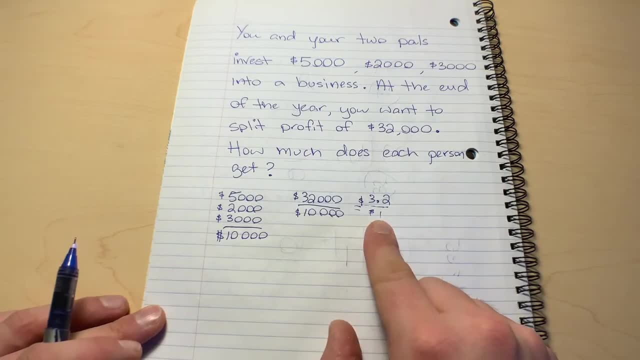 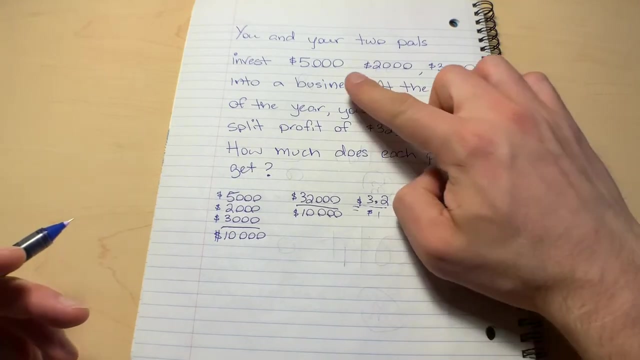 on the same line. right Bottom is $10,000 of investment. Once we divide, we get $3.2 for every $1 that someone has invested. So that's really the hardest part. Now we look at how much each person invested. Okay, well, 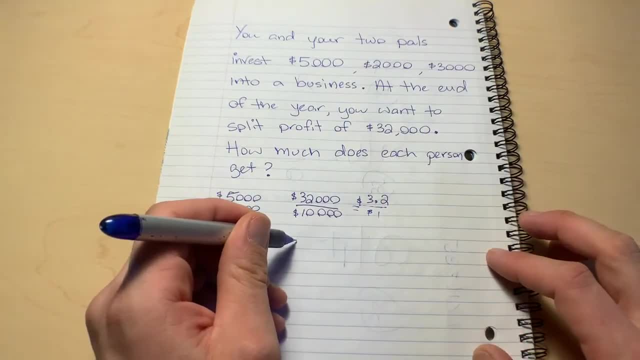 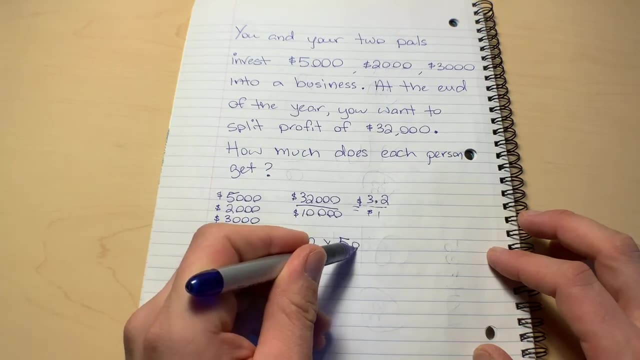 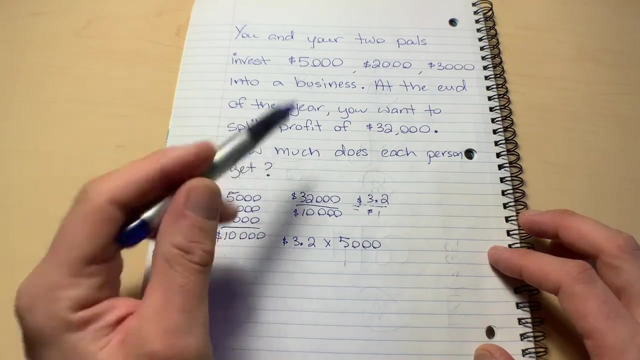 this person invested $5,000.. So we're going to say $3.2 times the first person's investment of $5,000.. The next person invested $2,000.. So we're going to go 3.2 times $2,000. 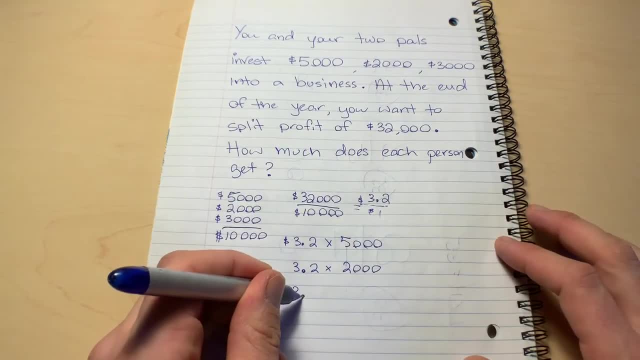 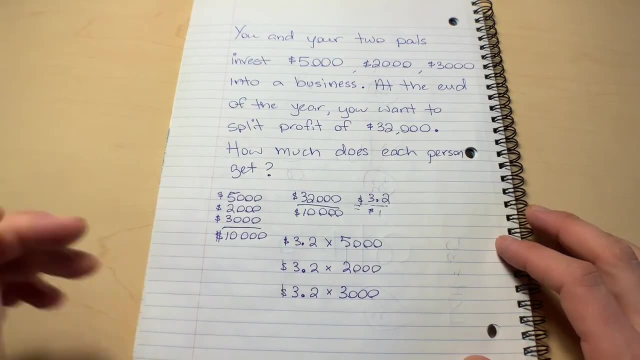 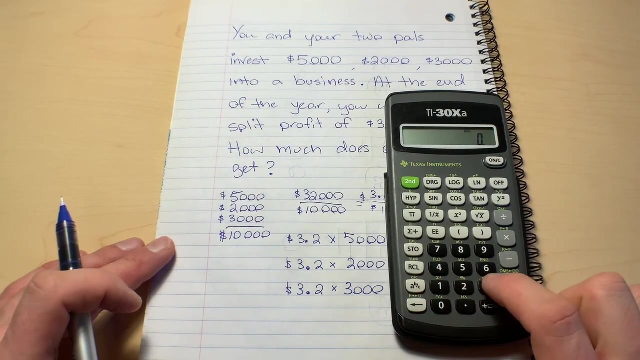 And the last person invested $3,000.. So we're going to go 3.2 times $3,000.. Okay, these are all dollars, Yeah, yeah, yeah, Okay, and when we multiply that, let's see what we get. here. I got my trusty old calculator And I'm going to go 3.2 times $5,000.